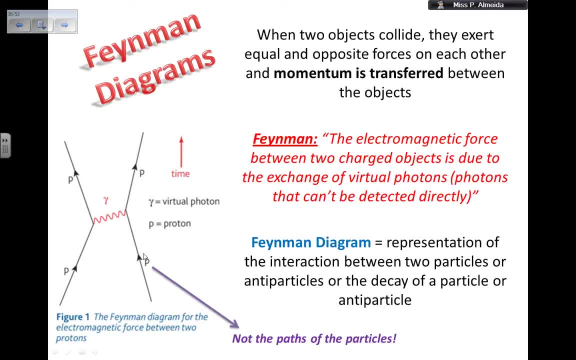 So this is before the two protons interact. This is after the two protons interact. The actual arrows: they do not represent a part of the particles, So it's just how I do it And in here in the middle, so kind of getting this type of shape together, I have the exchange particle. 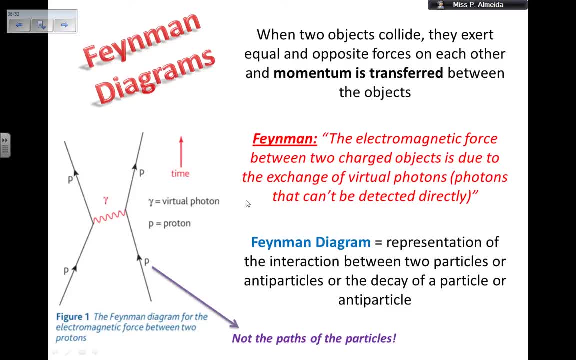 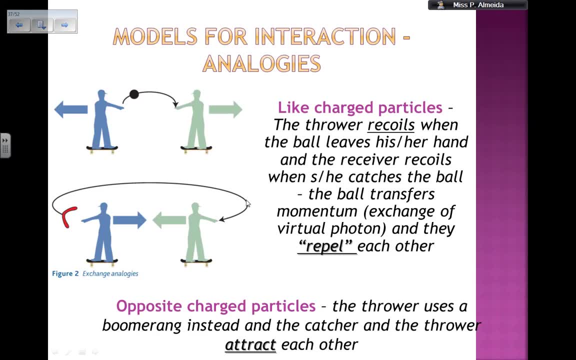 In this case I have a virtual photon Here. it is Because I'm talking about charged particles. You all know about other exchange particles later on. So this model is to explain why particles either attract or repel. So let's look at this diagram first with the blue guy and the green guy. 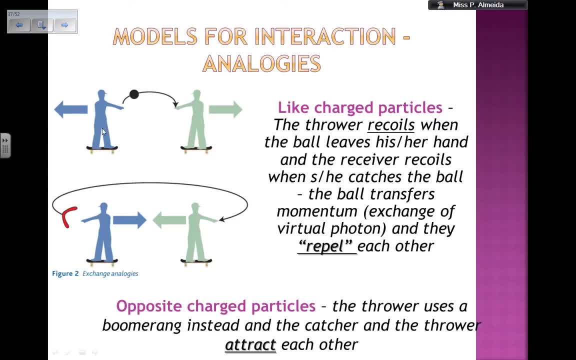 So like charged particles. So I have the thrower, the blue one. He throws a ball to the green guy Because momentum is conserved: as he throws something forward he moves backwards, So away from the green guy. So when the thrower recoils, that happens because the ball left his hands or her hands. 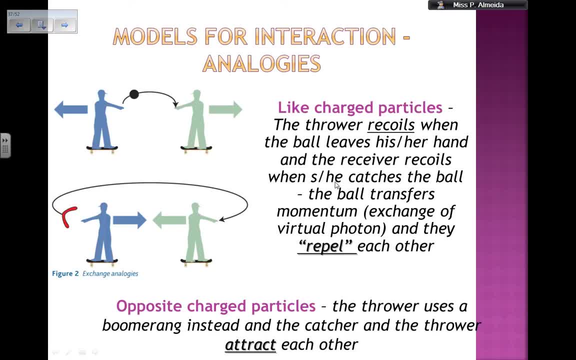 And then the receiver recoils when they catch the ball because the ball transfers the momentum, So kind of the exchange of the virtual photon, that exchange particle And they repel from each other. So this guy gets the ball moves backwards. They are like charges. 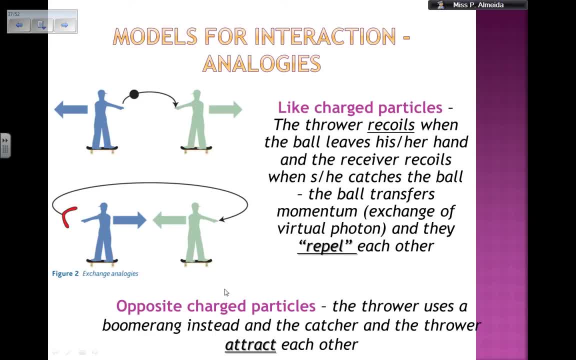 They repel Opposite charges, Then the analogy is thinking about a boomerang. So the blue guy is now throwing a boomerang to the green guy And because momentum is conserved as he throws the boomerang forwards, 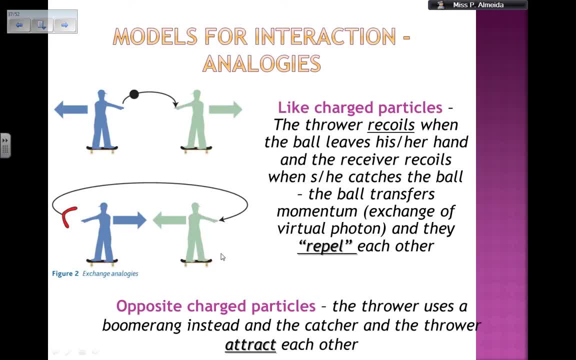 he goes backwards, getting closer to the green guy. The green guy receives the boomerang And because moment is transferred, he's going to go closer to the blue guy. So they attract each other, And that's what it says in here. 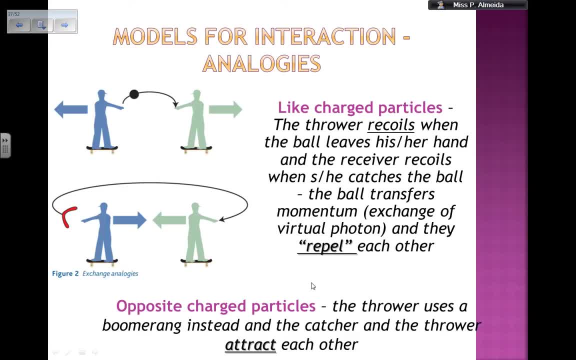 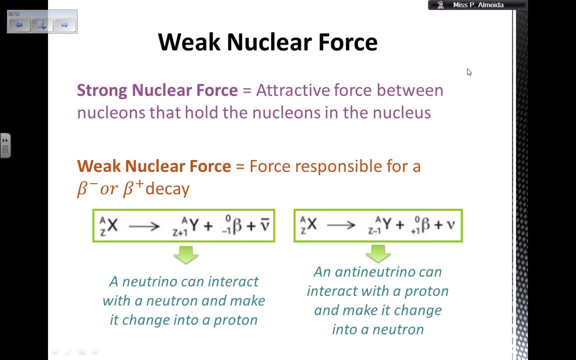 So opposite charged particles, The thrower uses a boomerang Instead, And the catcher and the thrower attract each other. Now, weak nuclear force. We need to know about the weak nuclear force Because it's going to be responsible for these decays that we are going to talk about now. 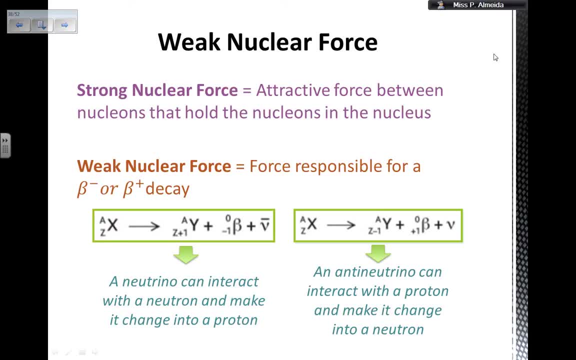 For these Feynman diagrams. But just make sure that we do not confuse the weak nuclear force with the strong nuclear force. I'm just giving you here the definition of the strong nuclear force that you got in the very first video, Which is called the structure of the atom, I think. 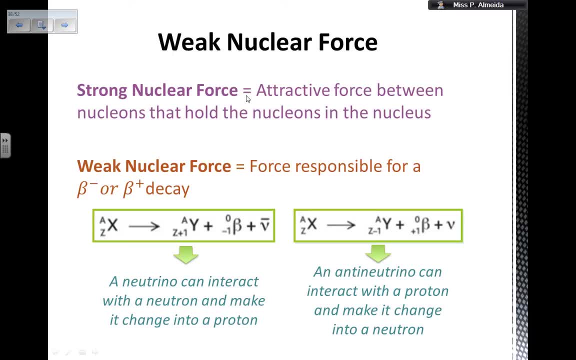 So the strong nuclear force is the attractive force between the nucleons, so protons and neutrons that hold the nucleons, so the protons and the neutrons together in the nucleus. I said protons and neutrons, right. 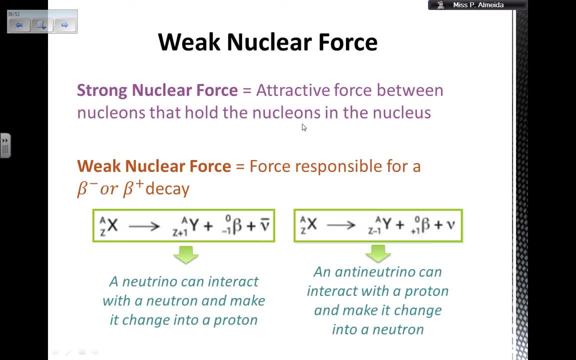 If I didn't. that's what I was supposed to say for the nucleons. A nucleon is how I refer to a proton or a neutron, So something that is inside the nucleus. So the strong nuclear force keeps all the protons in the nucleus. 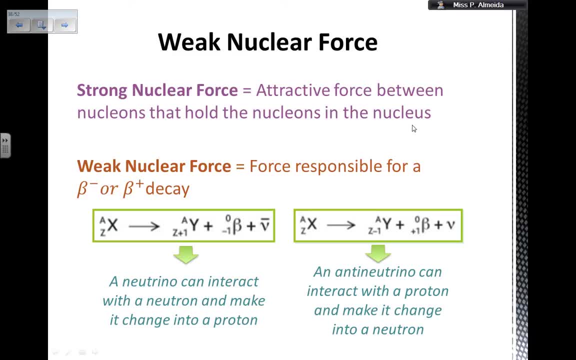 All the protons and the neutrons together in the nucleus. The weak nuclear force is going to be the force that is responsible for a decay, Either a beta decay or a beta plus decay, Which is standing for the positron decay. Look at the previous video, which is called particles and antiparticles, to see these decays. 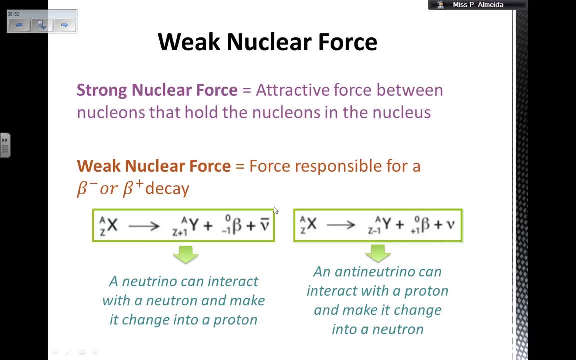 So this is the beta decay. So this one beta minus I have x, gives me y And I get a beta particle And an antineutrino. You may remember that this happens because I have too many neutrons and one becomes into a proton. 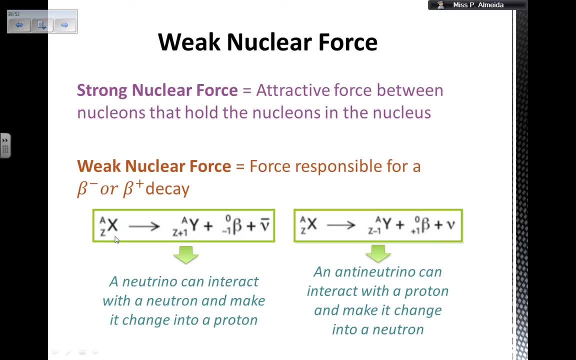 So in the nucleus I'm going to have this beta minus decay to happen because a neutrino- so nothing to do with this antineutrino- is a neutrino that is going to interact with a neutron. Remember that in a beta minus decay I have too many neutrons. 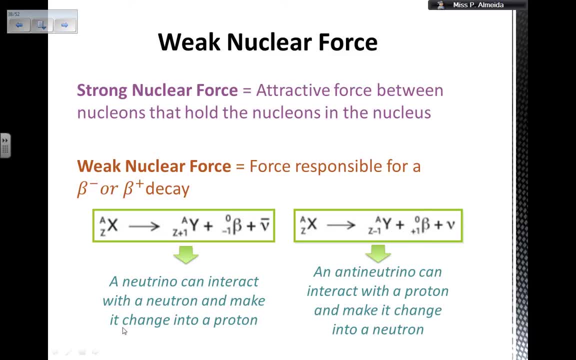 And it's going to make the neutron change it into a proton. So when I get a beta minus decay, I get too many neutrons. The neutron goes into a proton. This happens because of a neutrino. I get an antineutrino. 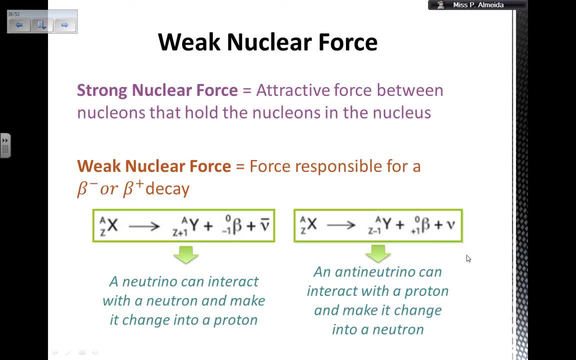 On the other hand, remember that I had in the last video the two decays, one next to each other, For us to make the comparison. So, on the other hand, if you understand the beta minus decay, you will understand the beta plus decay, really simply as well. 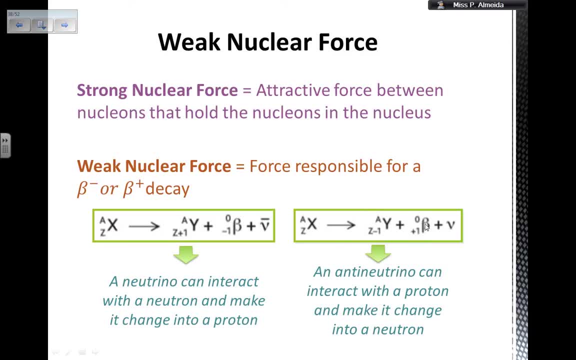 So in this case I have x gives y, plus the positron, The antiparticle of the electron, Plus the neutrino. So in the positron decay I have a nucleus that is too rich in protons And one of the protons is going to change into a neutron. 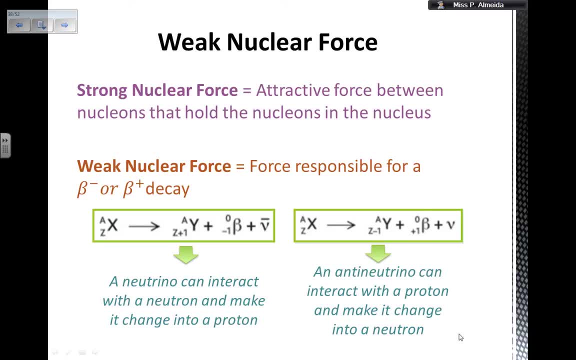 And I get a neutrino. So why does this happen? So an antineutrino is going to interact with a proton and make it change into a neutron, And therefore I get the beta plus particle and the neutrino. I know that I'm going a little bit too fast, but you can always pause the video. 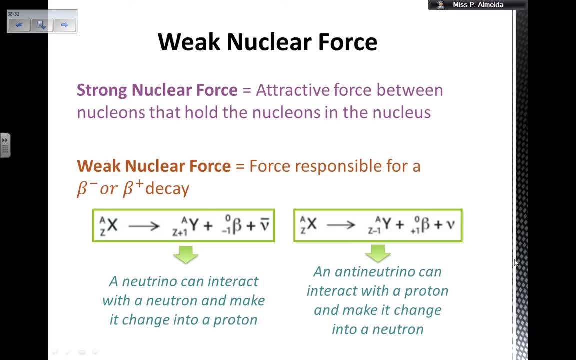 So weak nuclear force is the force that is responsible for these decays in the diagrams Beta minus. check in the previous video how it happens. The neutrino makes the rich in neutron nucleus. to get one neutron to go into a proton, I get an antineutrino. 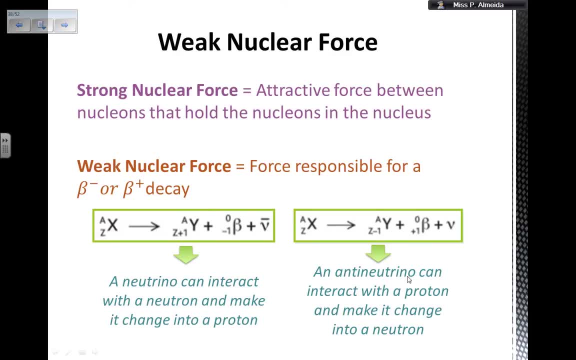 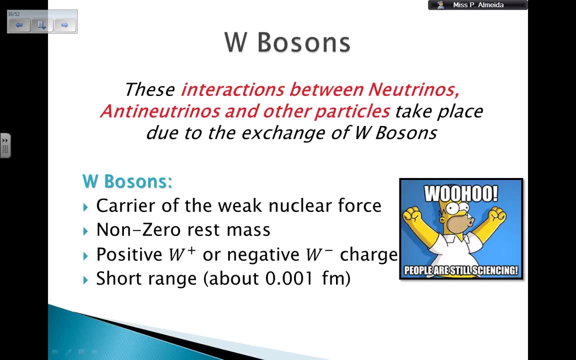 In the positron emission I have an antineutrino that makes a rich in protons. So I get a proton nucleus to have one proton to go into a neutron And when this happens I get a neutrino. So the W bosons, which are W standing for weak, 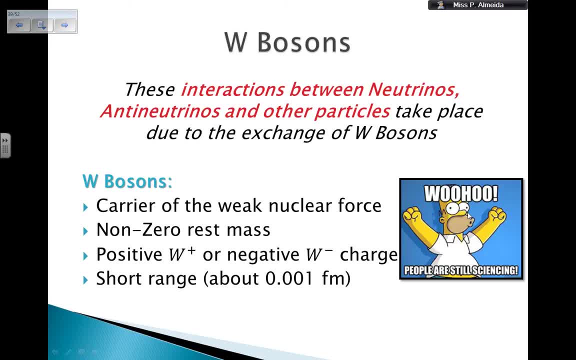 These are going to be the ones that are going to be responsible for these interactions. So these interactions between the neutrinos and the antineutrinos and the other particles, The neutrons, the protons, They take place because we are exchanging the W bosons. 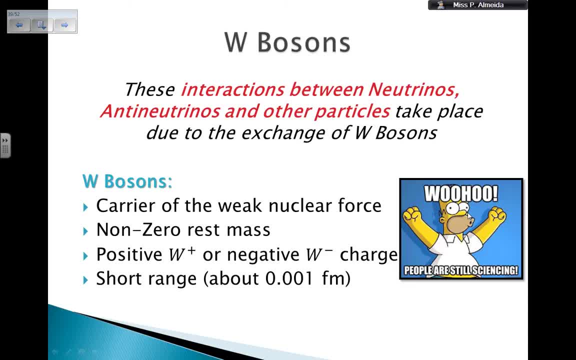 So for charged particles I exchange the virtual photon For antineutrinos, neutrinos and other particles, the kind of the coin that I use, So kind of, instead of giving money, or the chocolate. So the thing that I exchange to get something else from the other one is going to be the W bosons. 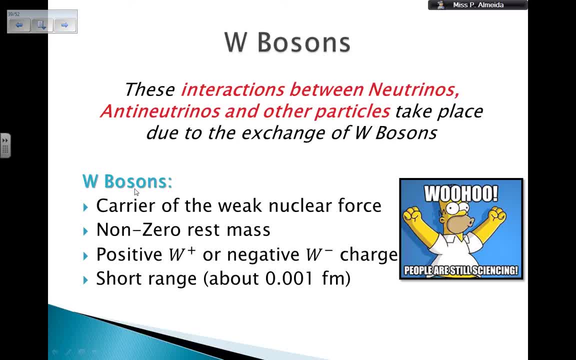 So the weak bosons, So W bosons. they are the carrier of the weak nuclear force, So they have the weak nuclear force with them. They have a known zero rest mass. They can be positive If I have positron decay Or negative if I have beta decay. 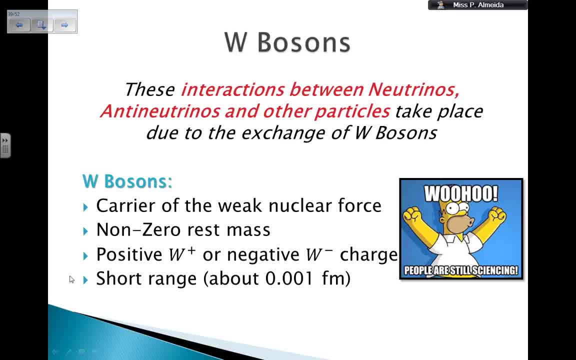 So they have this positive or negative charge And they have a very short range, So this happens only when things are very close to each other. So their range is about 0.001 fm, Which stands for phantometers, Which is 10 to the power of minus 15 meters. 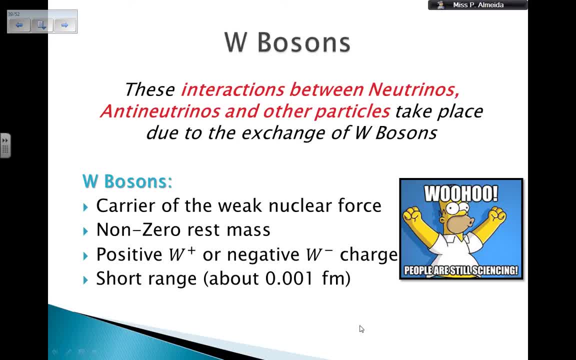 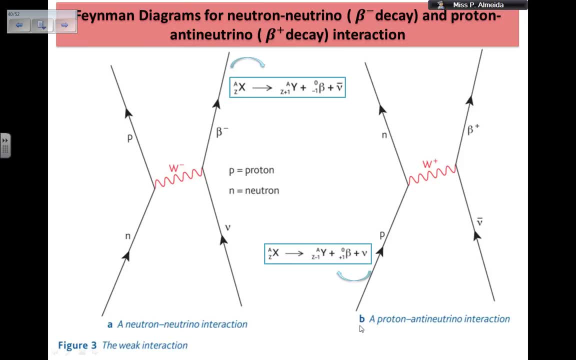 So again, this was The very first slide. Something like the structure of the atom, Or maybe actually it's in the second video, Which is the stable and unstable nucleus. Go on the videos and look for it. So Feynman diagrams for this interaction. 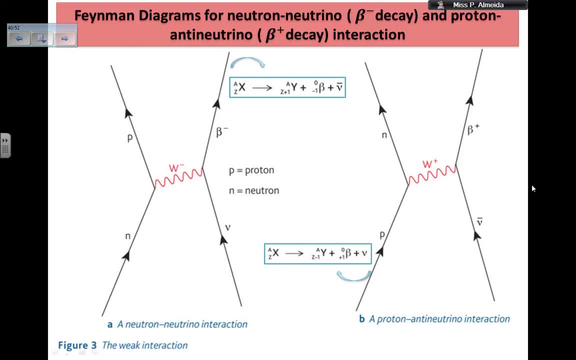 So I have here my beta decay and my positron emission. In terms of Feynman language, I can say that my beta decay is a neutron- neutrino interaction, Because my neutron is going to interact with my neutrino, Making my neutron to go into a proton. 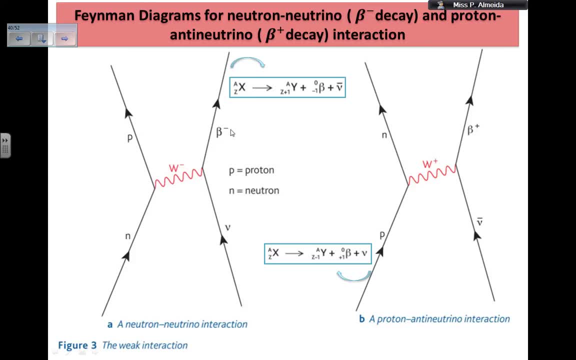 Look at the diagram And then getting a beta particle being emitted. So this is the representation of this equation In terms of Feynman diagram. I have a beta particle, So beta minus, So I get a W minus boson Now in the positron decay. 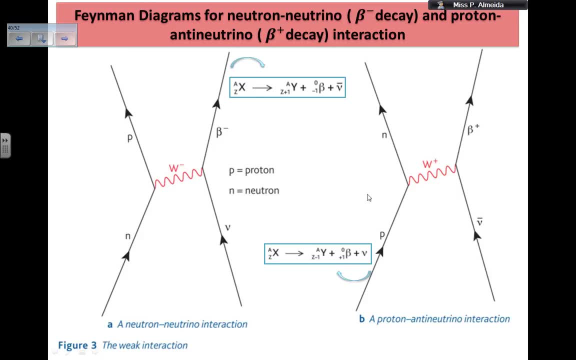 So when I have too many protons, One of them goes into a neutron. This is because of an anti-neutrino, So this is going to be In Feynman language. So in interactions, This is going to be a proton anti-neutrino interaction. 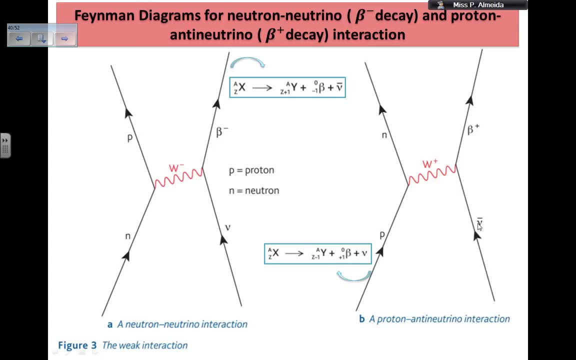 So again my anti-neutrino, Here we go. The neutrino symbol with a hat Meets the proton, Makes the proton change into a N Neutron And when this happens, I get a particle being emitted Which is. 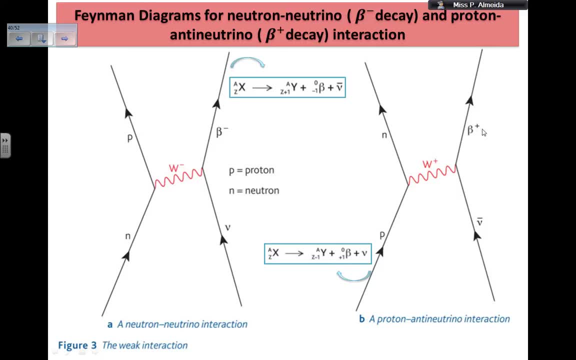 Here we go. The positron: beta plus, Again beta plus. So the W plus W boson, The positive one Gave me this interaction To happen, Okay, So made it happen. As always, The charge must be conserved. 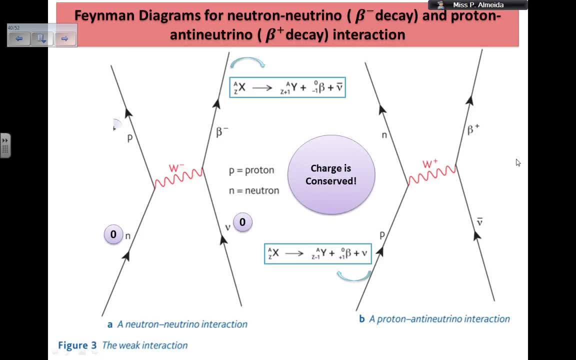 So let's see if this is working, So if this is making sense, If I want to see if my diagrams are correct, I can always think about the charges of the particles. If the charge is not conserved, It means that is wrong. 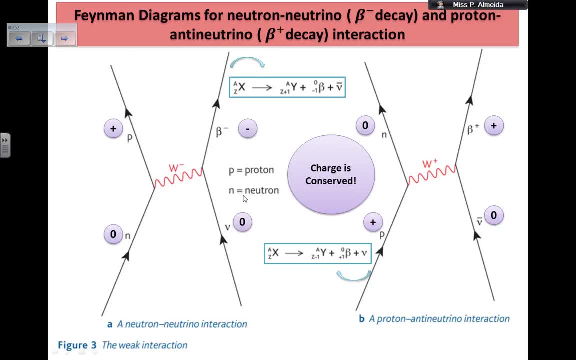 And we need to do it again. Okay, So charge before the interaction: Neutron zero, Neutrino zero. So charge before zero, And then after the interaction: Proton positive charge, Beta minus charge. So plus and minus, I get zero overall. 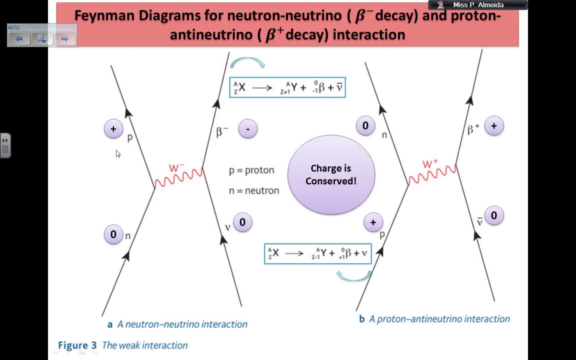 Overall. Sorry. So zero before, Zero after Charge is conserved. Let's look at the other one. I have a proton positive charge Meeting an antineutrino zero charge. It gives me a neutron positive charge And a positron positive charge.